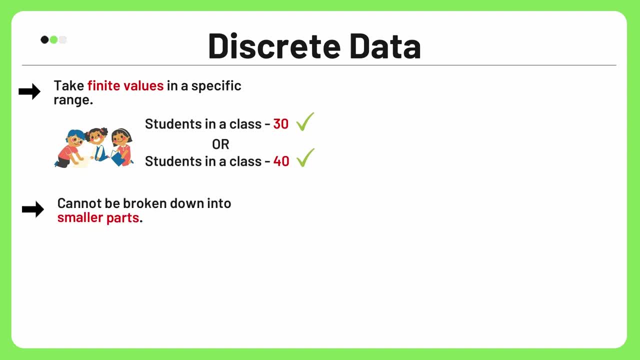 specific range for each school. Discrete data cannot be broken down into smaller parts to make them more precise, and it is nearly impossible to measure between two fixed values. Example: the number of students in a class cannot be broken down into fractions, That is. 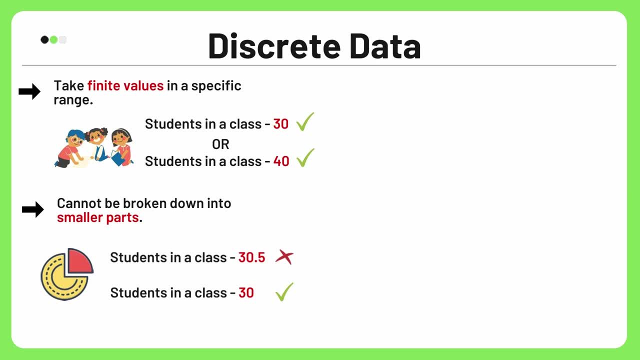 we cannot say that we have 30.5 students in a class. Discrete data consists of distinct or unconnected elements which are non-continuous in nature. For example, let's assume class A has 30 students and class B has 35 students. Clearly, 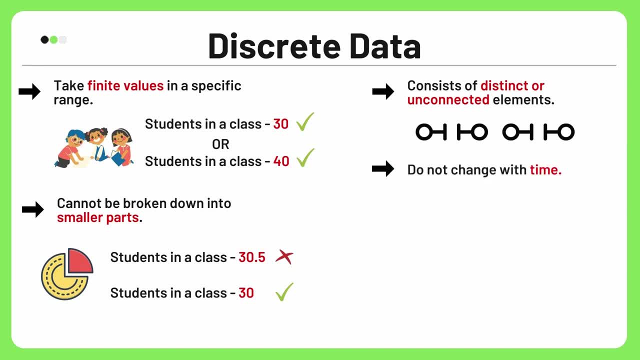 both the counts are unrelated to each other. Discrete data generally do not change with time. Example, the number of students in a class will not change every month. Under statistical data analysis, discrete data can be easily visualized using bar charts or pie charts. If discrete data 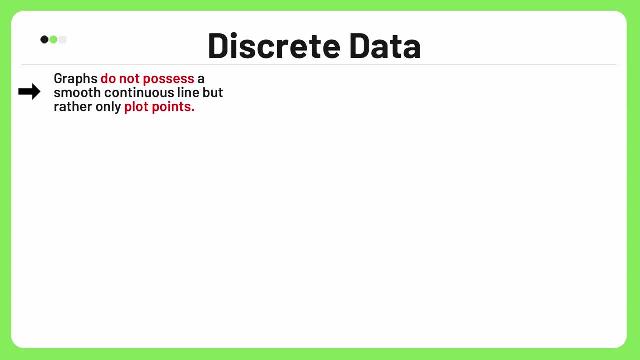 is a line chart, then the graph represents value at specific points along the number line. These graphs do not possess a continuous line, but rather only plot points above consecutive integer values. Discrete data is counted and is not measured. Example: you can simply count the number of. 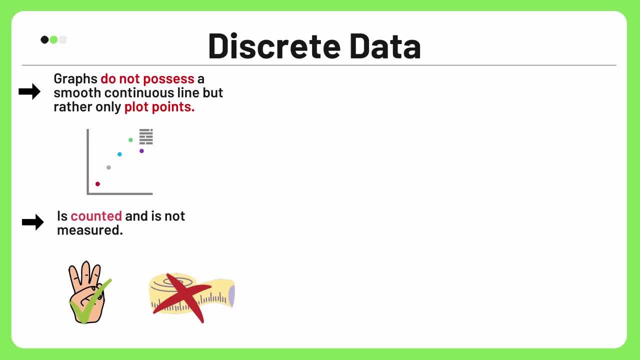 students in a class instead of measuring it using a measuring device. Discrete data can be whole numbers, like the count of students in a class, or they can also be any other fixed number type, eg shoe size, shoe size, class size, shoe size. 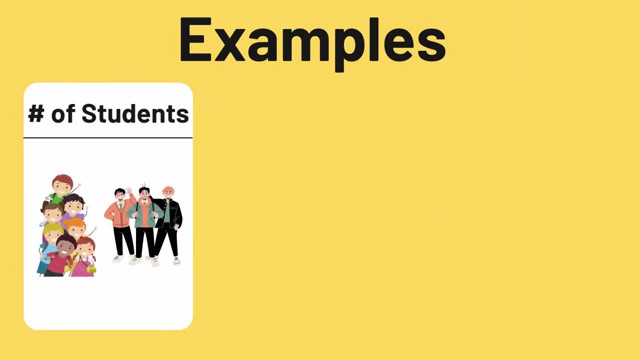 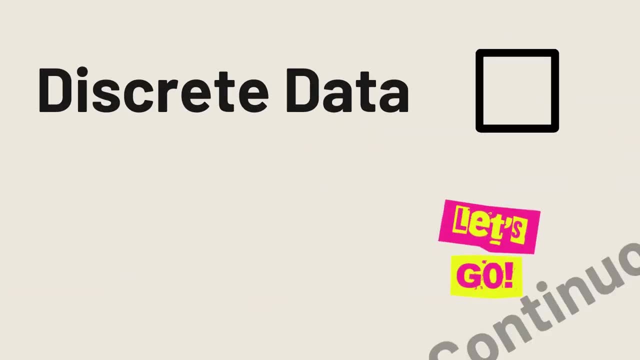 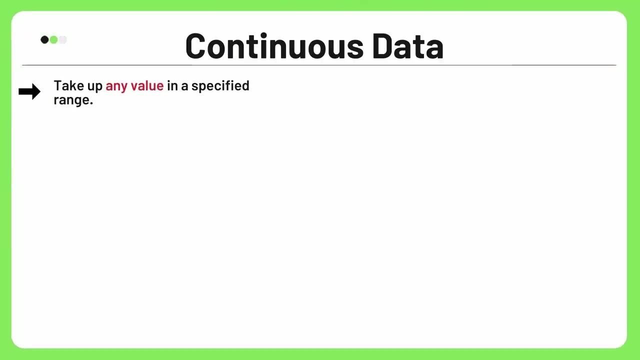 3 or 3.5.. Some examples are number of students in a class, number of tires in a vehicle and shoe size. Now that we know about discrete data, let's explore continuous data. As the name suggests, continuous data can take up any value in a specified range. We'll 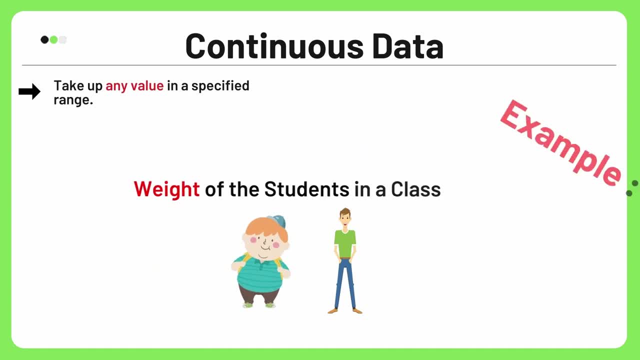 consider an example of the weight of a student in a class. The weight of students in a class can take any value from 30 kgs to 100 kgs. Continuous data can be broken down into smaller parts to make them more precise, based on the sensitivity of the scale, For example. 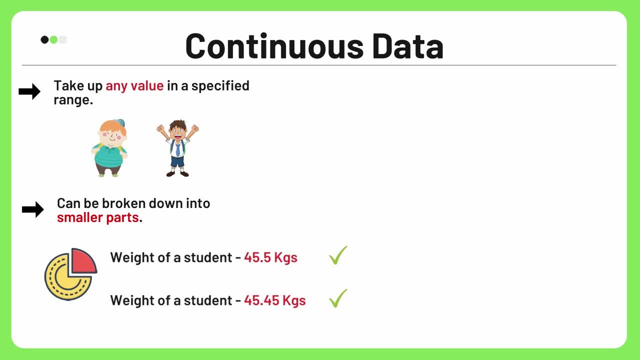 the weight of the students in a class can be fractional as well, which means that one student can weigh 45.5 kgs and the other student can very well weigh 45.45 kgs. This type of data consists of connected elements which are continuous in nature: Continuous data.